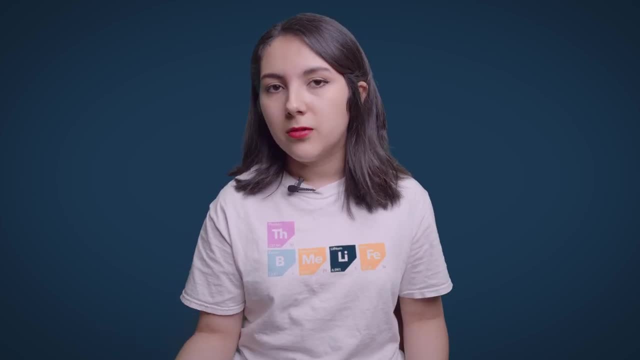 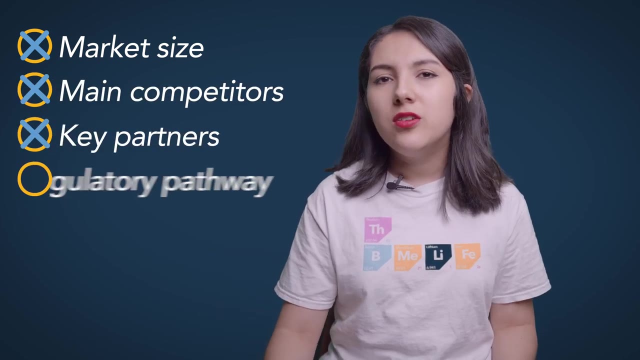 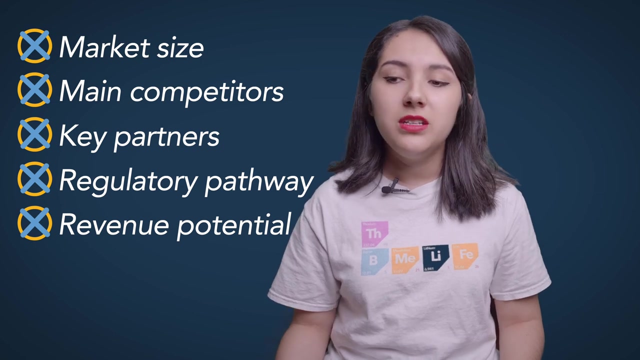 actually going to benefit as a company creating this product. Look at the market. Who are our biggest competitors, which are probably Colgate Crest? We look at what kind of regulatory pathway would we enter. We look at what is our potential revenue. So we need to be realistic of how much. 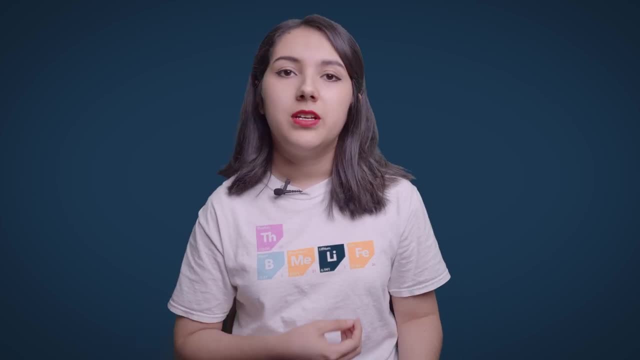 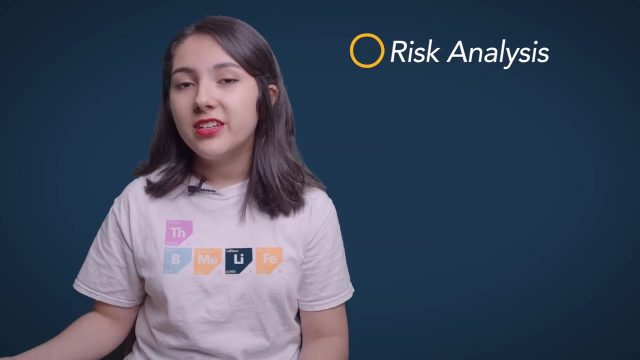 this could actually benefit. What is the cost? How much money are we going to ask from investors? How much are we getting back? What is our timeline? It's probably many, many years. What is the risk of us failing? Also, if our product is a novel product that has never been, 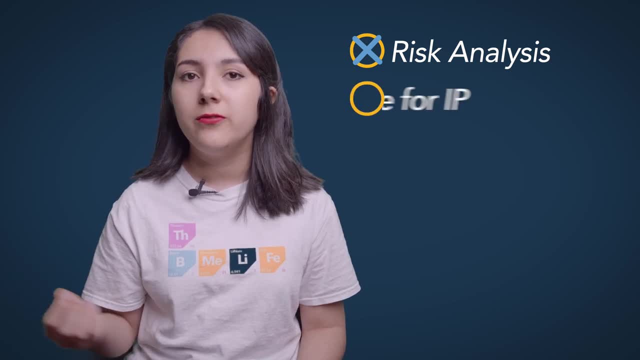 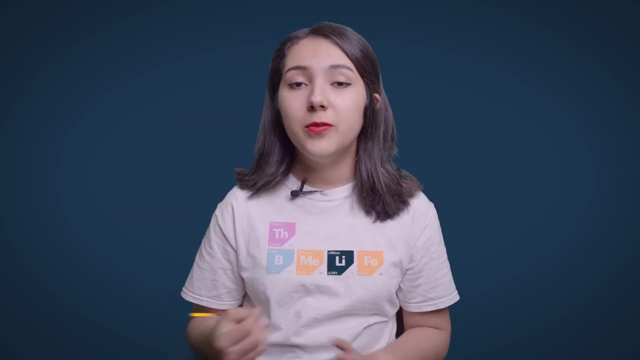 seen before. we would probably want to file for an intellectual property patent To make sure that no one copies our product. The next phase is formulation, concept and feasibility. We already assessed the risk, assessed the market, and now we're going to be. 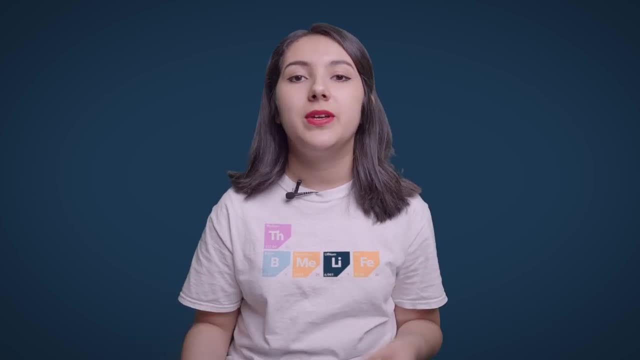 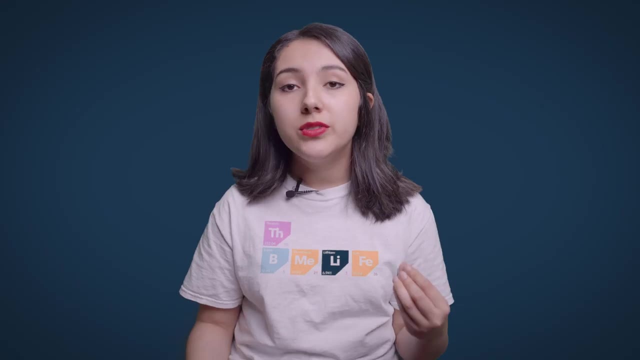 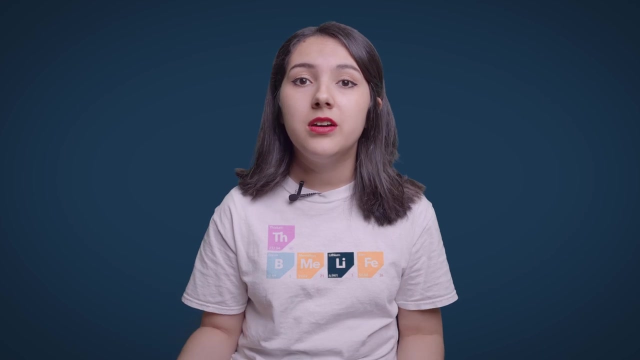 looking at what is our device going to look like. We have to start prototyping, designing. We have to start all the solid work, drawings. We have to choose the materials that we're going to use, choose the manufacturers that are going to be building our device, start thinking of assembly. 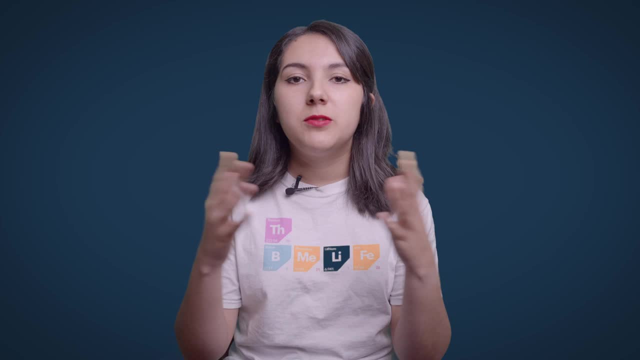 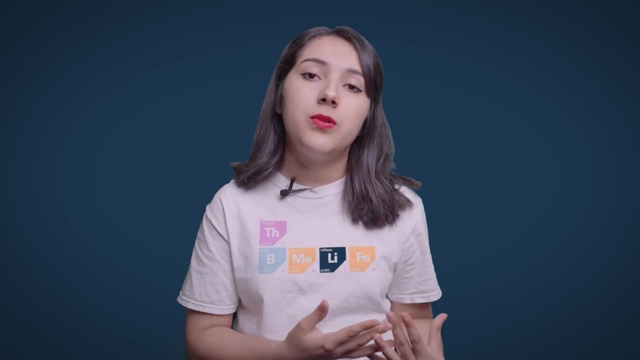 protocols, and then we're going to be looking at what is our market potential? Are we going to be looking at what is our product going to look like? We have to start conceptualizing our device and what it's going to look like. Our design is going to be driven by the customer requirements that we 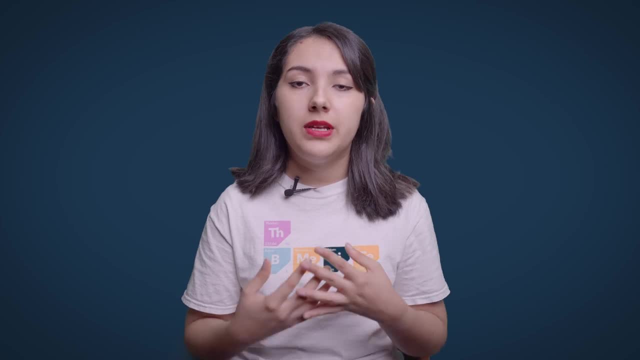 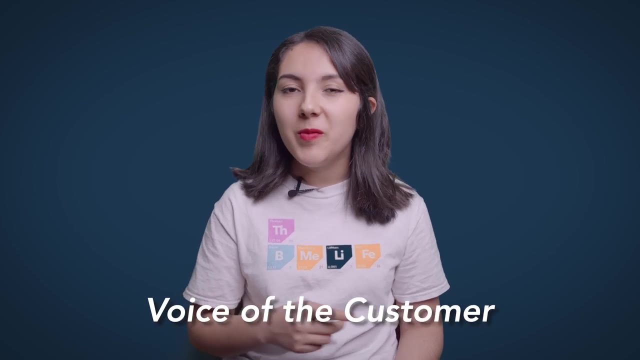 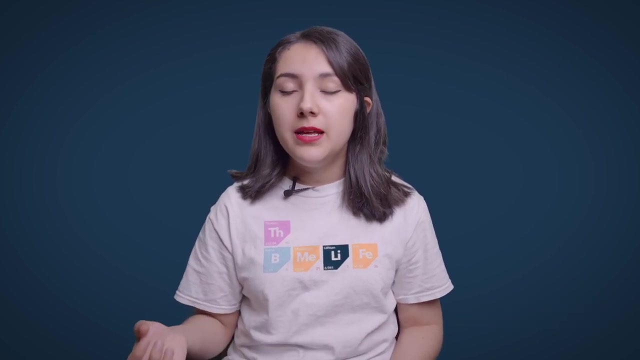 got from the dentist, the customers that we interviewed and things like that. In this phase, it's very important to listen to the voice of the customer. If you're a biomedical engineer, this is a term that you should know. It's really important to listen to what they want and implement it into. 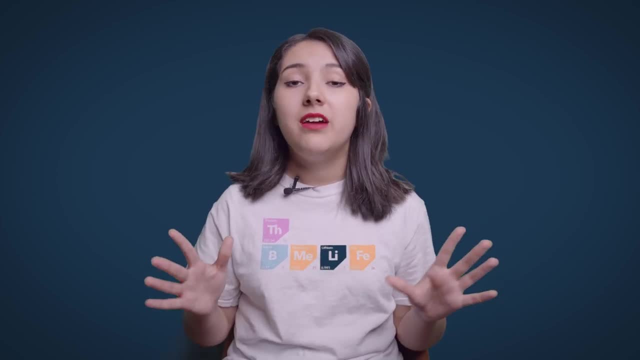 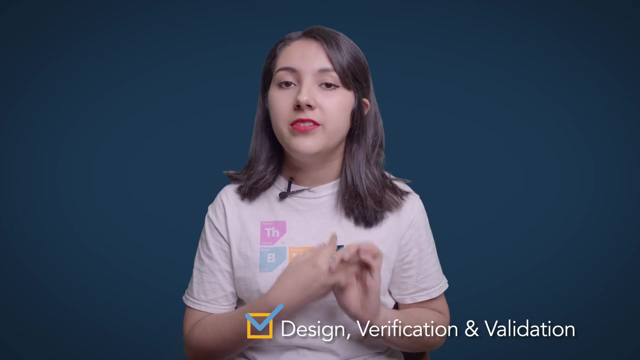 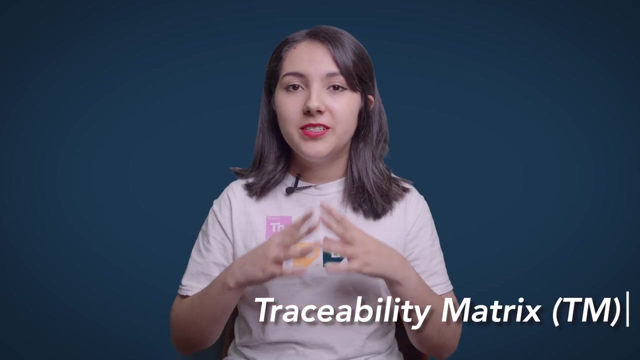 by interview, surveys or research. Now that we have our device and its design, we can enter the design, verification and validation phase, also known as V&V. To start, what is usually done is creating a traceability matrix. A traceability matrix is basically the blueprint of your device. 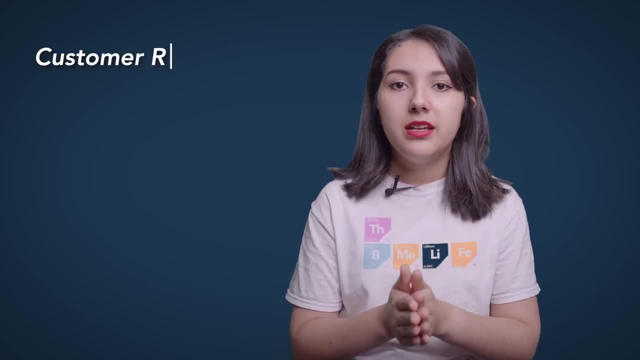 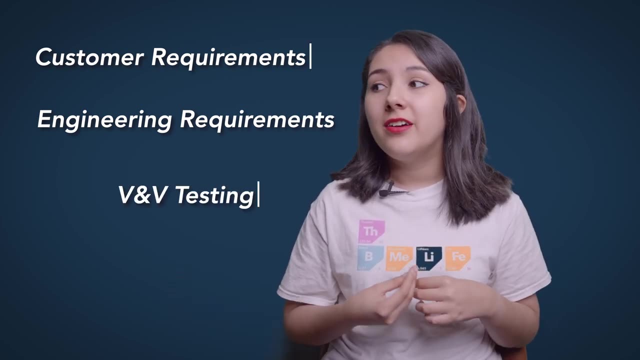 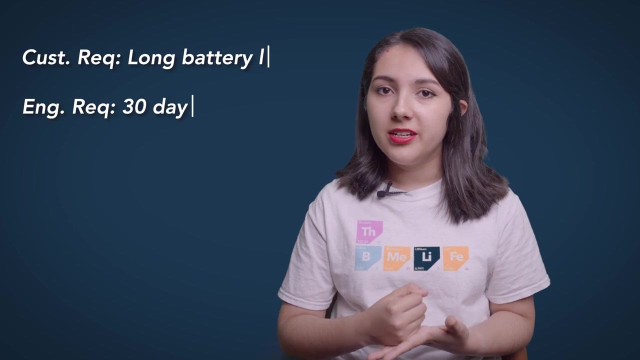 and how it meets the customer requirements. that were translated into engineering requirements, which are then verified by testing. So, for example, we mentioned- we mentioned that our customer wanted a long battery life for the toothbrush and we as engineers, we said: we're giving 30 days, But you need to create a testing protocol to how you're. 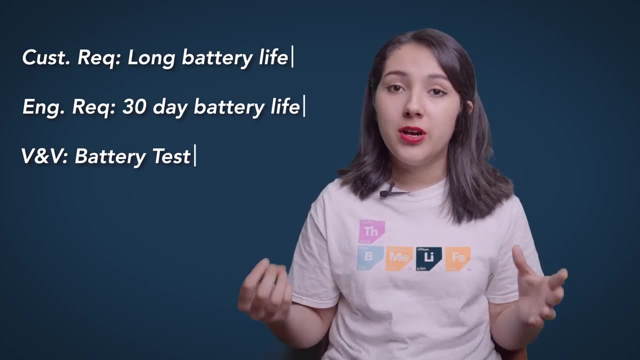 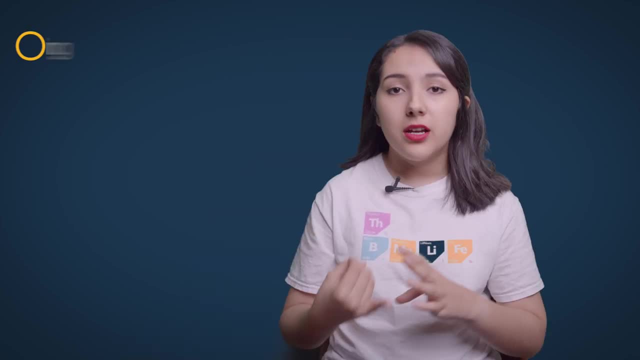 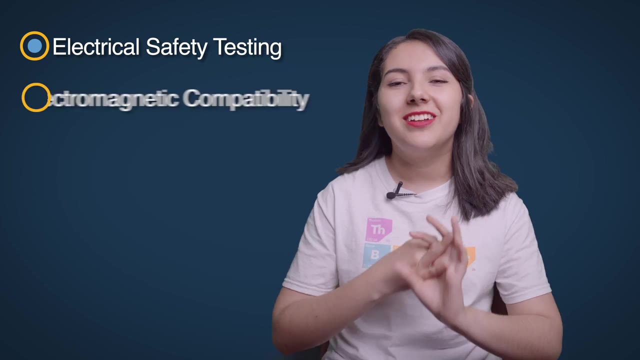 going to be testing that and all the other requirements that drive your design. Other tests that also go along with verification include tests such as electrical safety testing, which all electrical devices have to go through to verify that they're safe for the user. Electromagnetic. 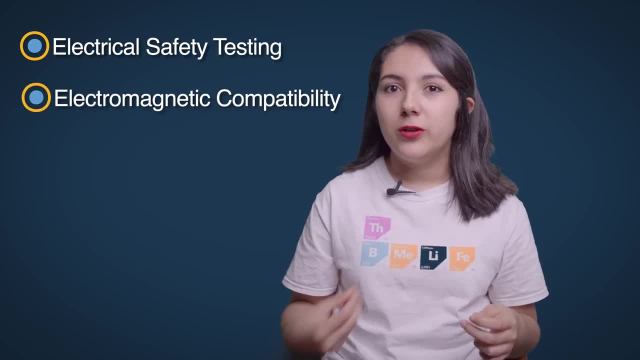 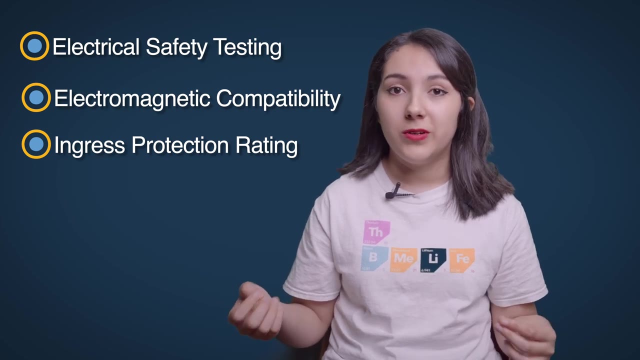 compatibility testing to verify that, you know, things like frequencies from the phones or just things around us will not interfere with the performance of the device. And then there's also IP rating testing to verify that no fluids or solid particles will interfere with the performance. 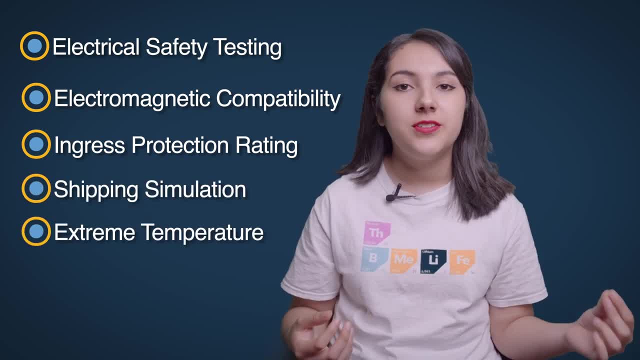 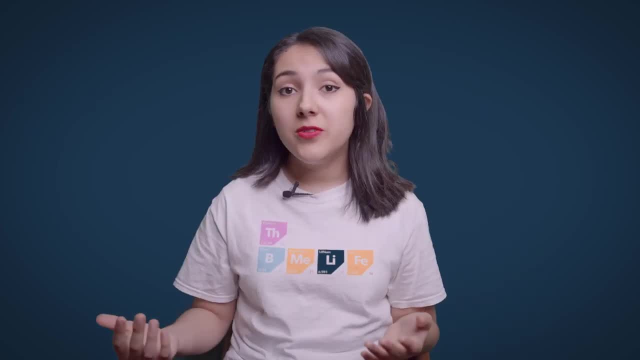 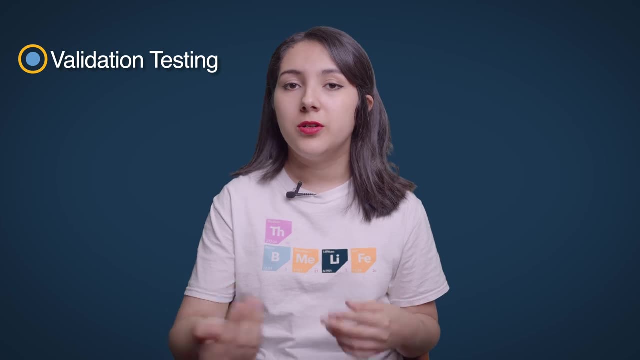 There's also shipping simulation, extreme temperature simulations, just to verify that your device will endure things like storage or shelf life, for example, And along with verification, we mentioned that we have validation. So this is where we bring the device to the customer and we ask them: does it meet your requirements and your needs? So this is where 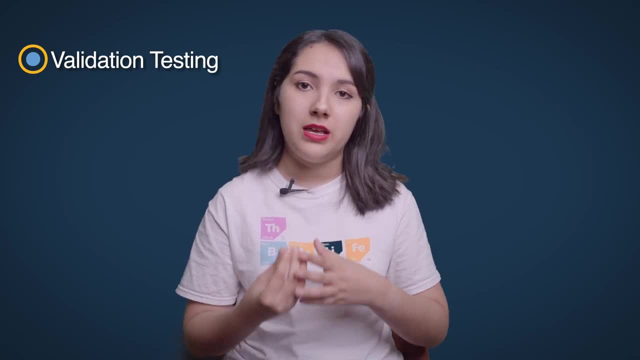 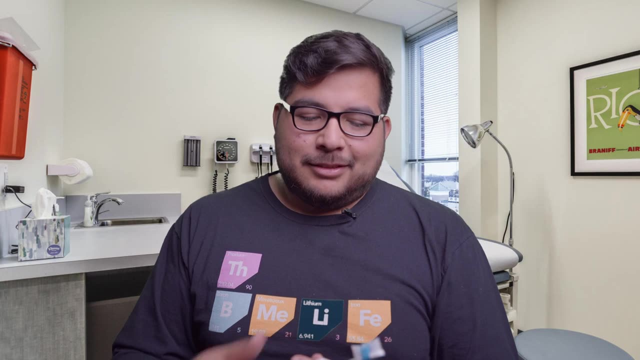 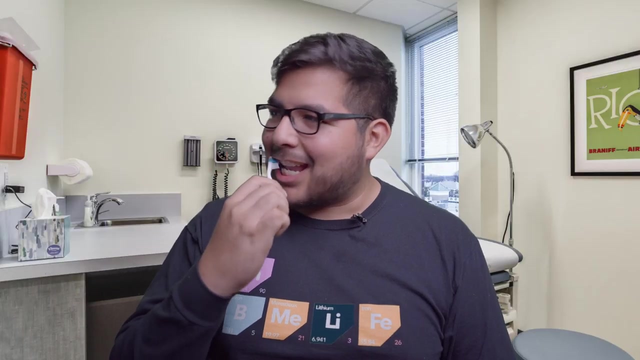 the customer comes in and they say: yes, this device does what I wanted to do. Adrian, does this toothbrush 2020, meet your needs? I don't usually like toothbrush or toothpaste, but hey, is actually. i like this. this is perfect. this is exactly what i wanted, everything i was looking. 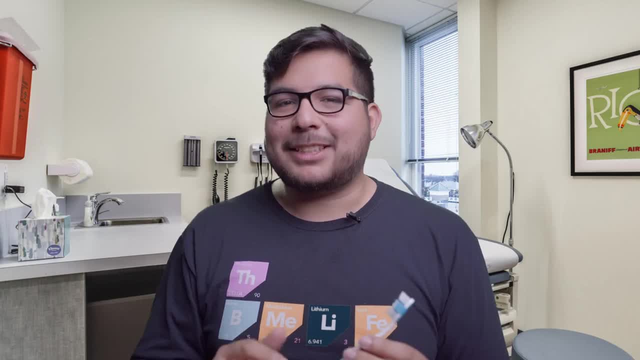 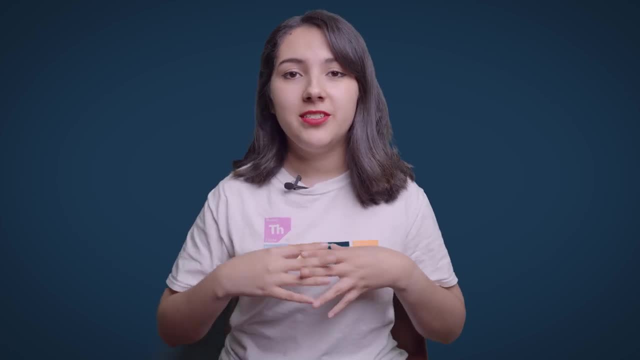 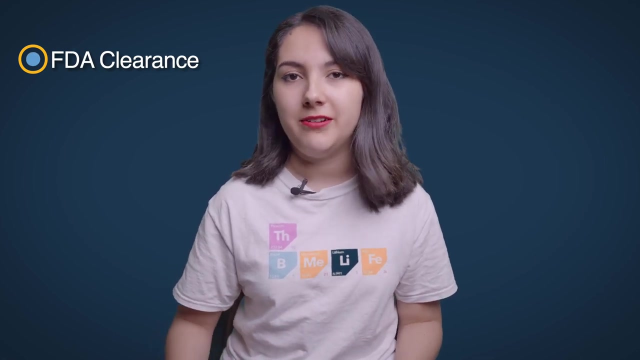 for in the toothbrush. this is amazing. thank you so much. now remember, while we're gathering all these tests and data, we are collecting all the information needed to file to the fda to get clearance in our device. we cannot go into the market until we get fda clearance and the fda 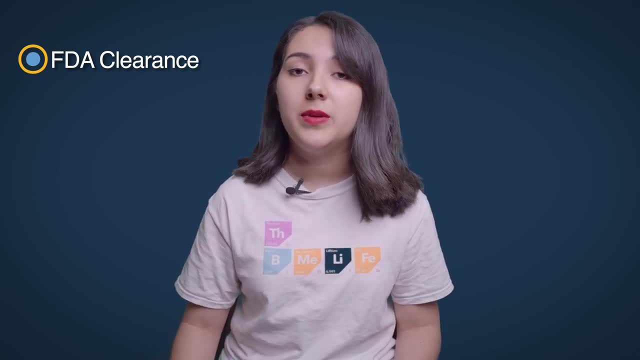 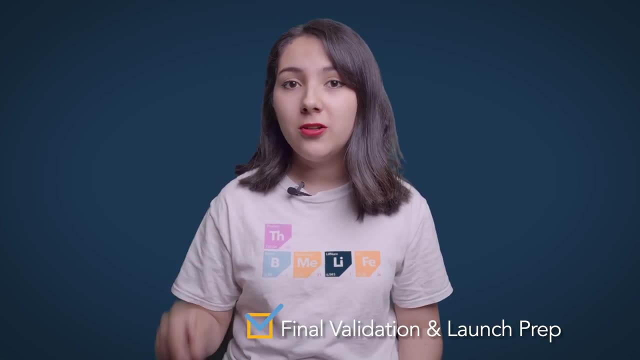 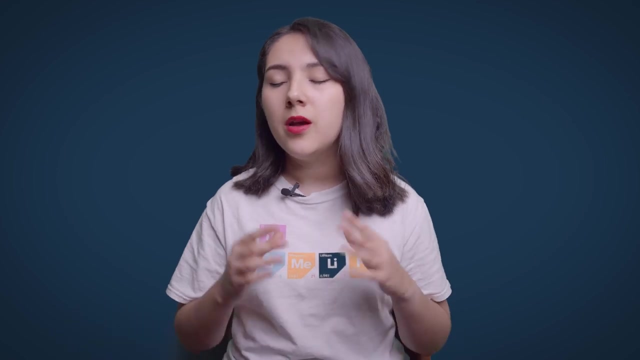 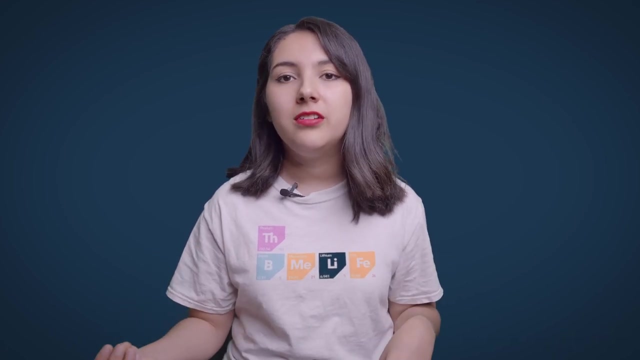 actually requires for three months of testing data to be able to complete your submission. now phase four is final validation and launch preparation. so you're finishing up all your tests, all your biocompatibility, electrical safety performance testing, shipping testing, packaging testing, all the tests, you're gathering all the necessary documents for fda submission. 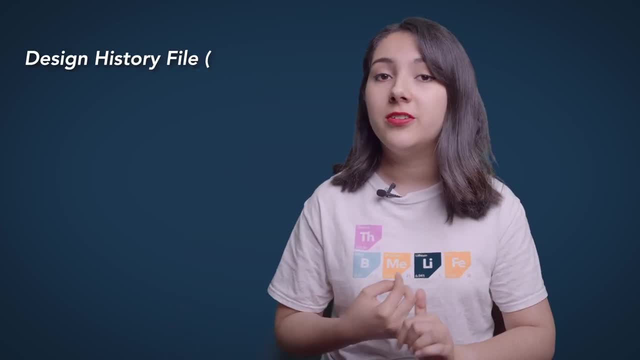 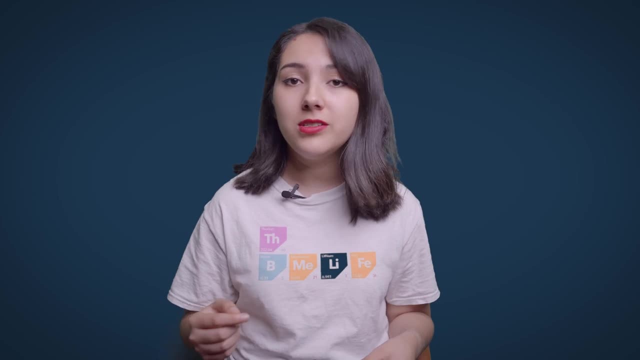 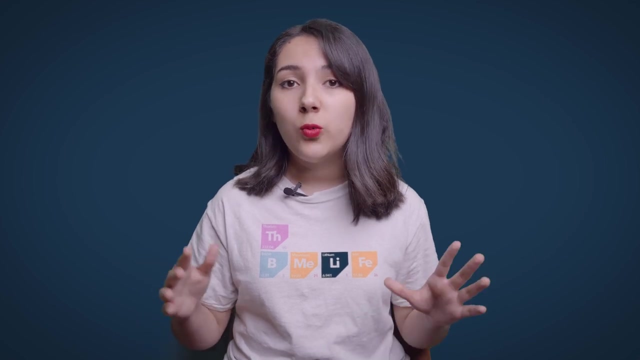 such as your design history file, your your device master record, a description of your device. you also need to take into consideration that once you get fda approval, you're going into the market, so you want to have enough products to sell once you enter the market, so you need to make an analysis of how many. 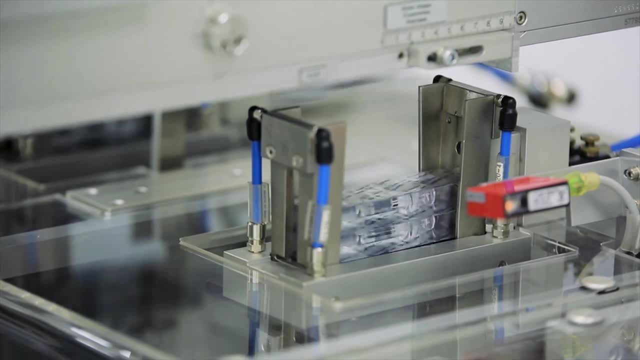 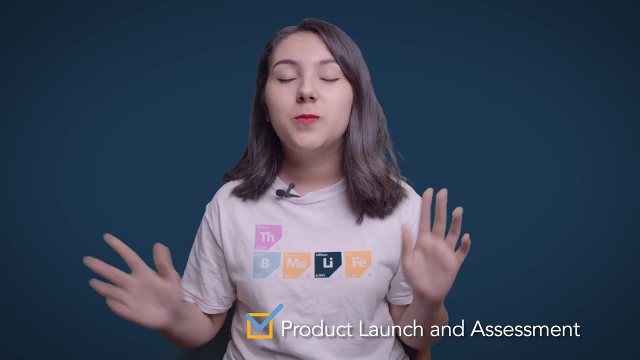 products you would expect to sell, how much you have to scale up in your manufacturing and have all those products ready to go, and the final phase is facelift. so the final phase is facelift, which is product launch. congratulations, your toothbrush. 2020 was. 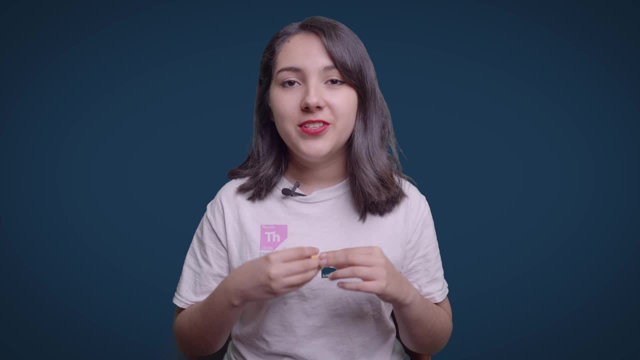 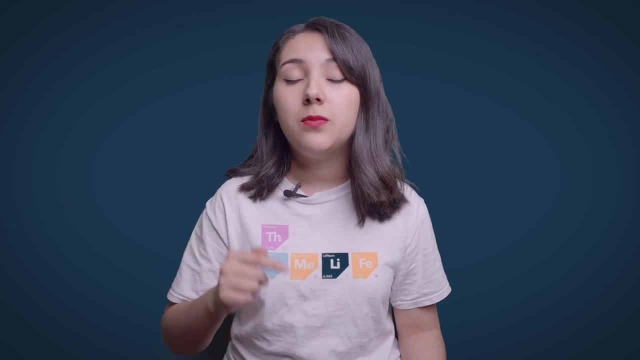 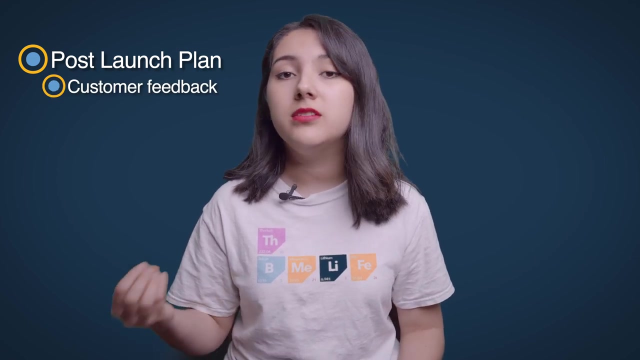 fda cleared, you can now sell it and you can start making revenue now don't forget that once you go into the market, you need to have a post product launch or post-market plan. how are you going to acquire feedback from the customers that you can implement into your device for maybe gen 2 designs? 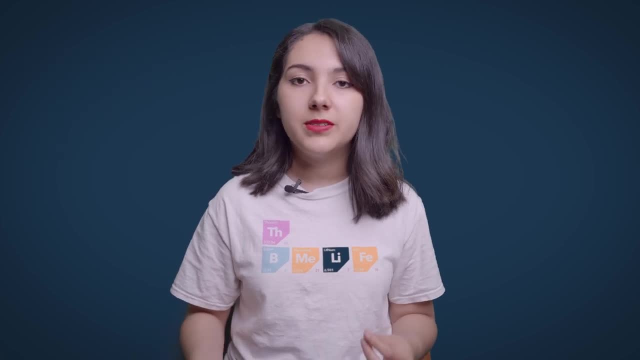 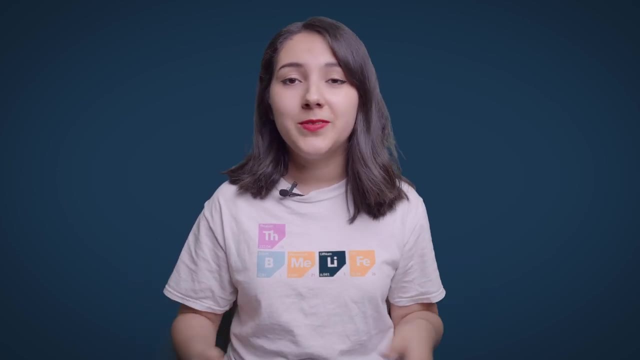 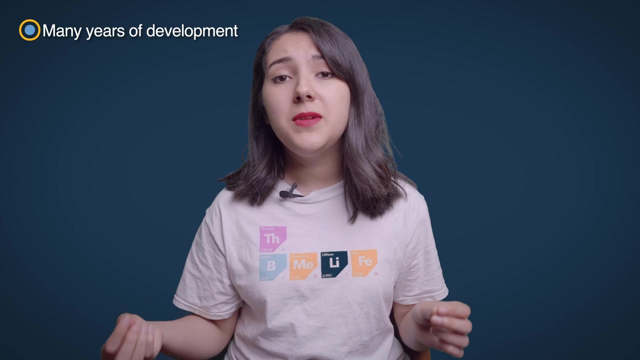 or just for continuous improvement of your device. now, one thing that we must not forget is that we are a startup. this whole process probably took us about 10 years from our initial idea to the final market approval. this means that we probably needed a lot of money for funding, probably. 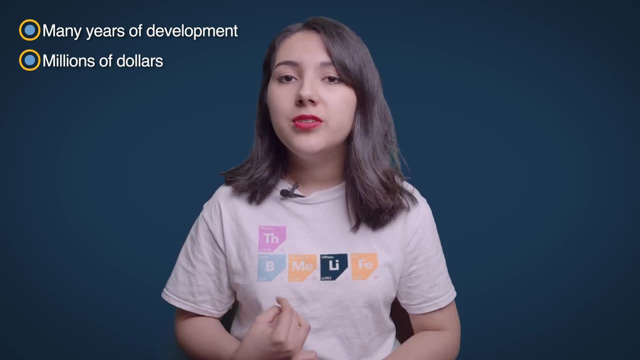 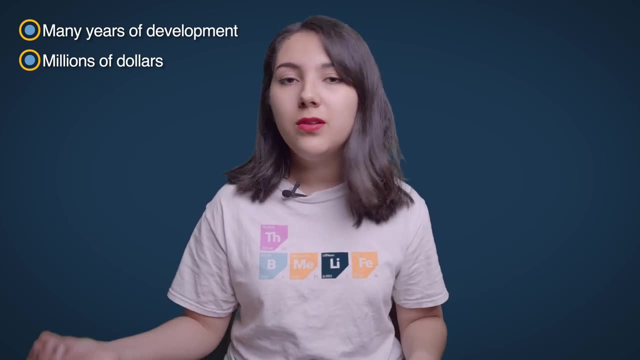 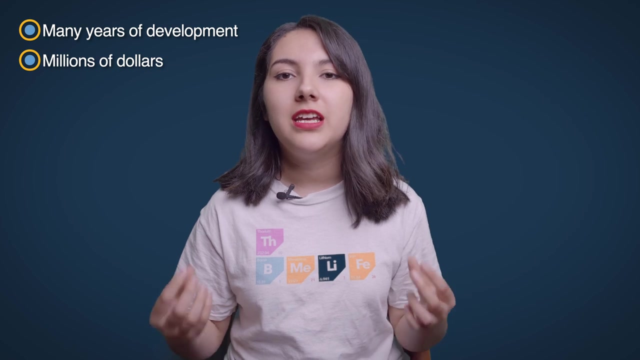 millions of dollars, not only for manufacturing or prototyping, but also for all the other costs like testing, rent everything, employees, your own salary. everything is money. time is money, so you needed a good series of funding in the beginning. where did you get this fund from? probably investors, we. 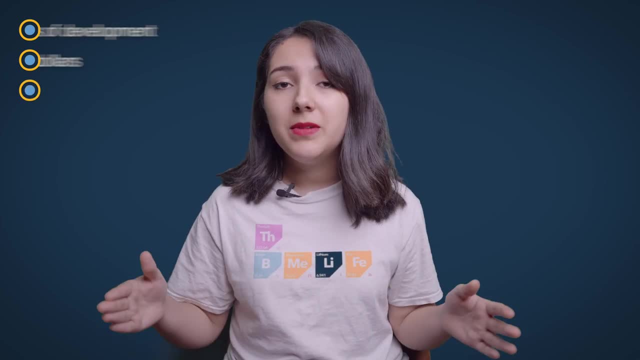 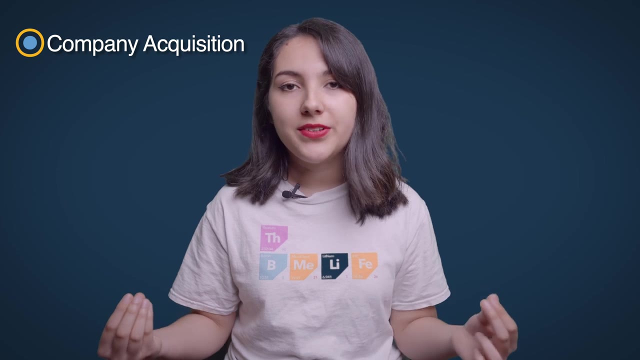 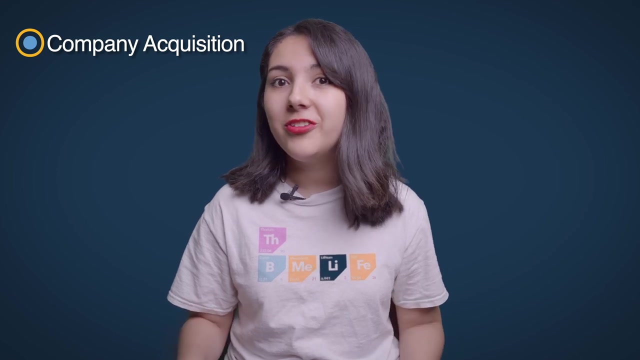 also have to take into consideration that at any time now we probably will get acquired by a company, like we mentioned before, like colgate or crest. so now that our product is approved, all this time along, colgate and crest have had us under their microscopes. they've been looking at us and our 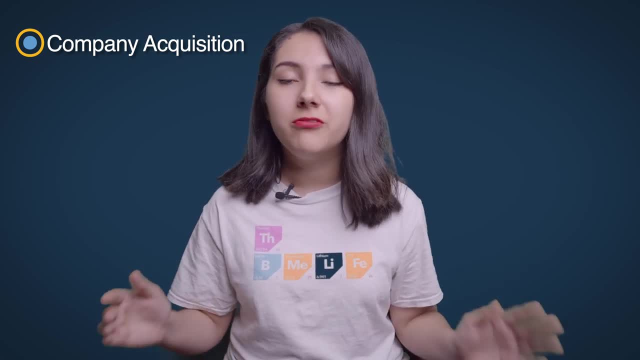 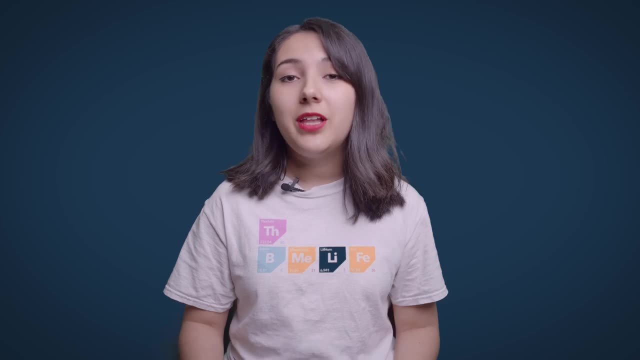 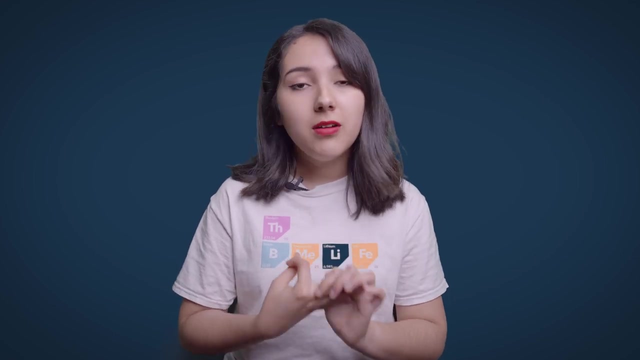 development and now that we're approved and risk free- well, maybe not risk free, but definitely low risk company- they are interested in acquiring us. like i mentioned, we had investors in the beginning, we have the founders and if we have any employees, they probably all have shares and once.